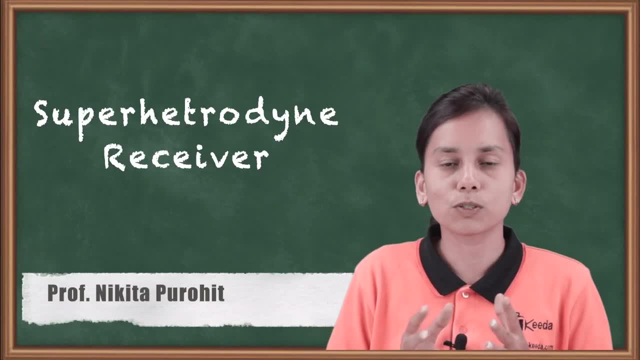 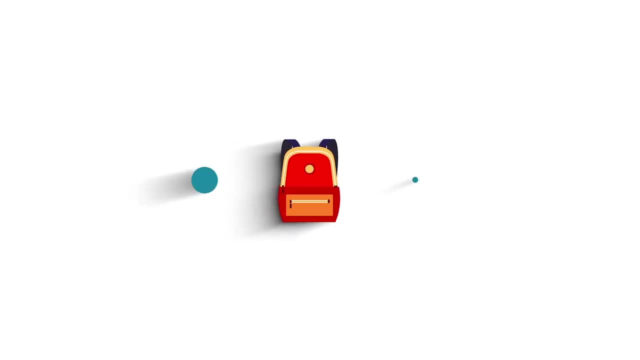 Hello friends, in this video we are going to talk about super heterodyne receiver and the whole process of receiving in the super heterodyne receiver. If I am transmitting a signal which is actually transmitted with the help of any channel and after travelling through the channel, it will receive by some receiver. 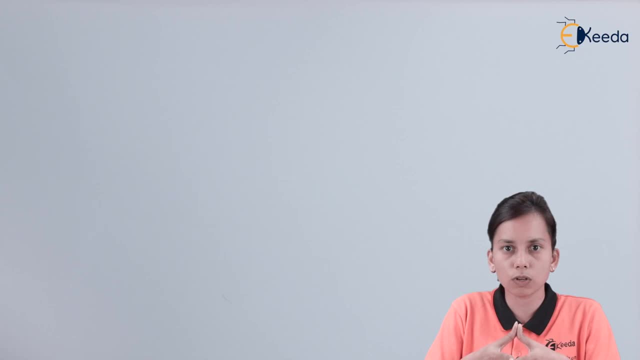 So what we are basically going to do in this whole session is to understand that. what is the procedure of receiver, how it is converting the received signal into our actual form. First of all, whenever we radiate the signal or we are transmitting the signal, it is in a form of electromagnetic wave. 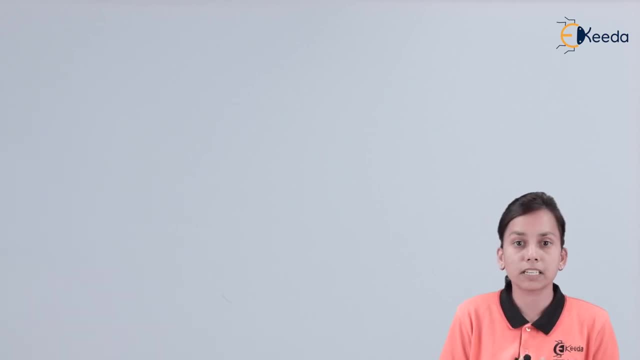 So our receiver will accept that particular signal, that electromagnetic wave, then it will process the signal and then it will give us the desired or the wanted form of a signal. Let us look at the block diagram of the super heterodyne first, then we will discuss it one by one. 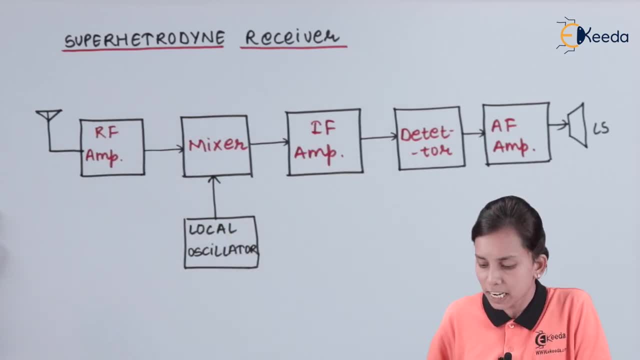 So this is the block diagram of the super heterodyne receiver. It consists of RF amplifier- this is our antenna- RF amplifier, mixer, oscillator, then IF amplifier detector, AF amplifier- loudspeaker. This AF amplifier stands for audio frequency amplifier. 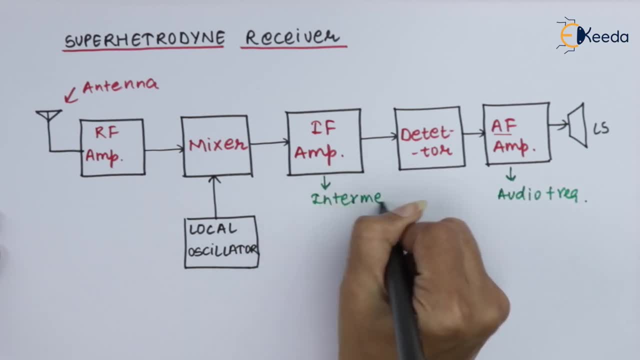 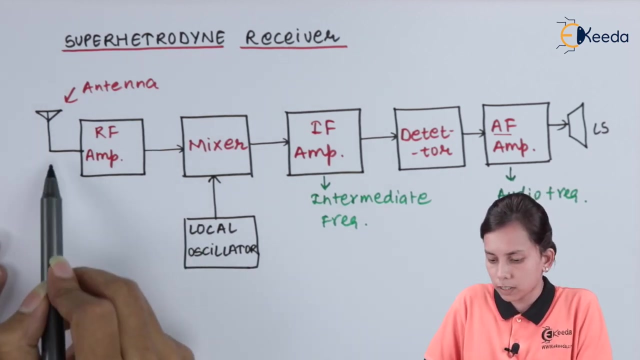 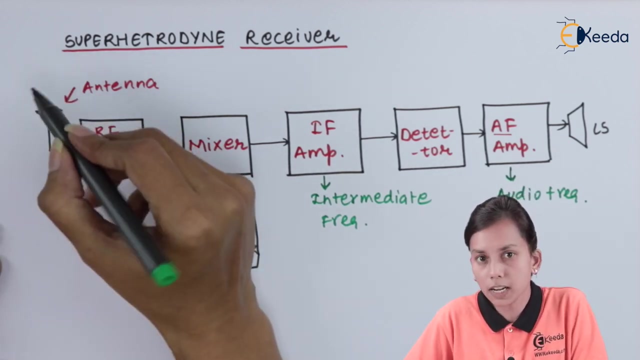 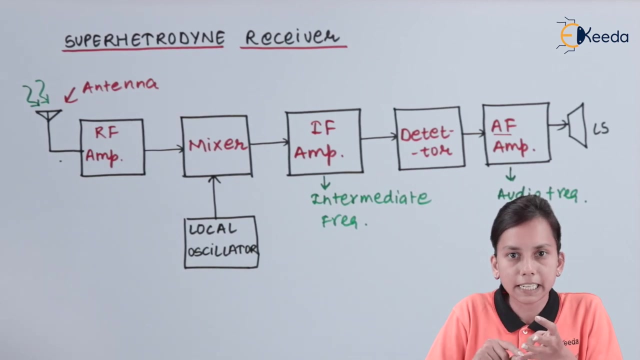 IF stands for intermediate frequency amplifier. So let us start our discussion. First of all, the receiver, First step of the receiver is antenna. This antenna, So let us say antenna is receiving the signal or the electromagnetic wave. So what we can say? that antenna is accepting the electromagnetic wave. 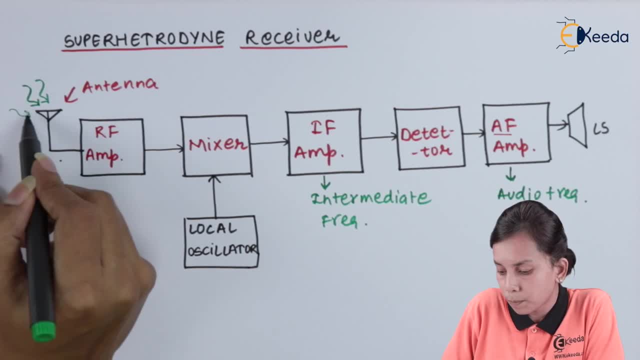 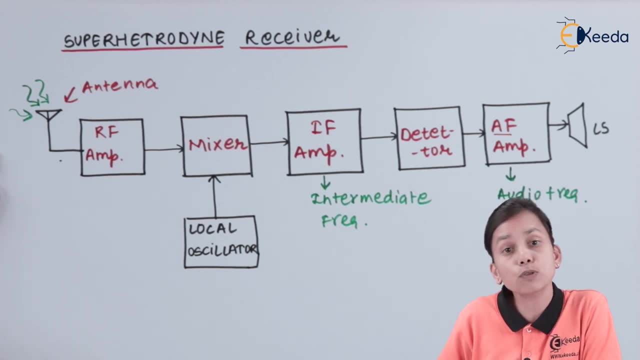 This antenna, when it is accepting the signal, it can be of various frequency, because we don't have a single radio station, We have so many radio station. So the function of antenna is to accept the various types of frequency. So how we can summarize the function of antenna. 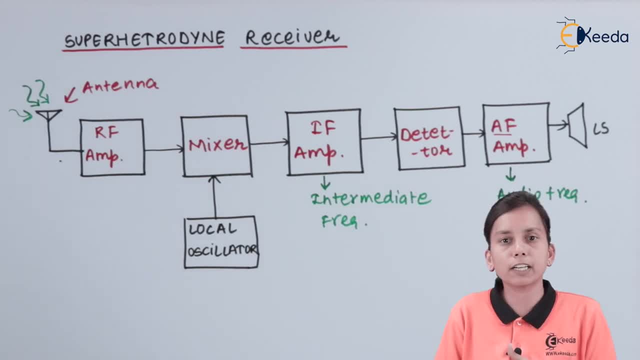 First one, that antenna will accept the electromagnetic wave of different frequency and then it will process to that electromagnetic wave and convert it into a electrical wave. So what I can say: that electromagnetic wave is converting into electrical wave. So we have two function: accepting the electromagnetic wave. 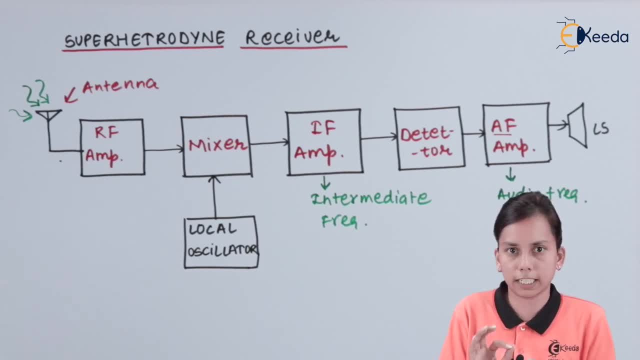 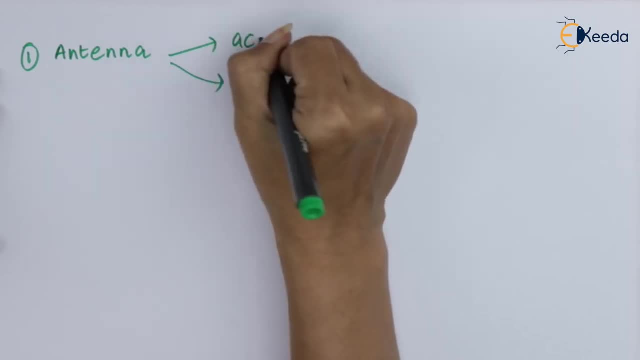 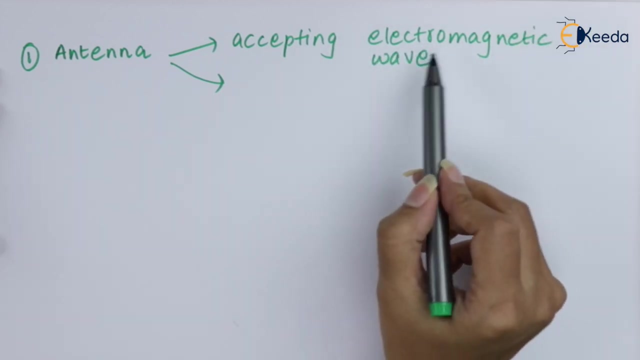 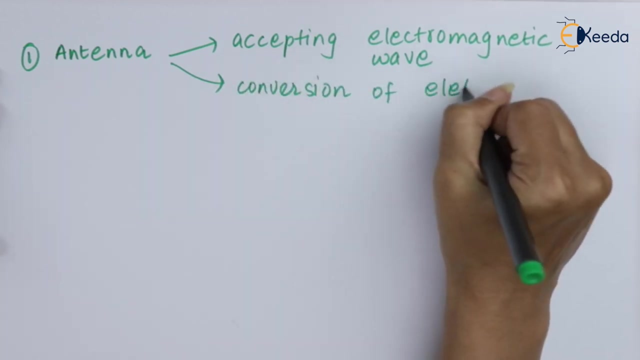 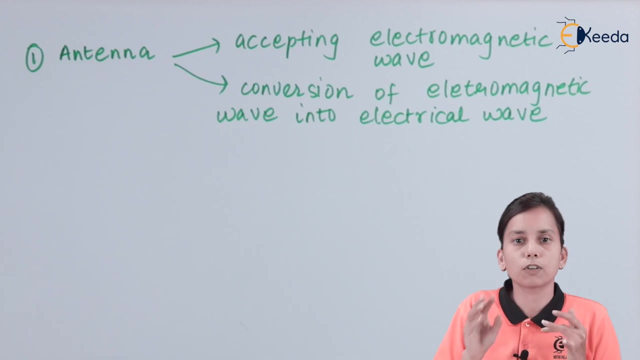 conversion of electromagnetic wave into electrical wave. Let me write down this point: Accepting electromagnetic wave of various frequency And second point, Conversion of electromagnetic wave into electrical wave. Now, one of the most important point for the antenna is that it is accepting electromagnetic wave. 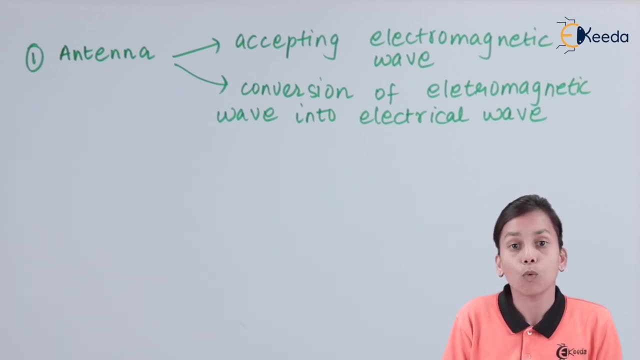 But it do not know that. what should be my frequency? For example, I want to accept the frequency of 98.3 kHz- This is how I tuned my receiver- But our antenna is accepting 98.3,, 98.4,, 98.5.. 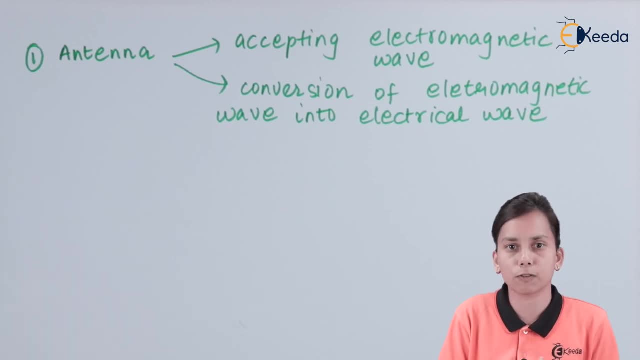 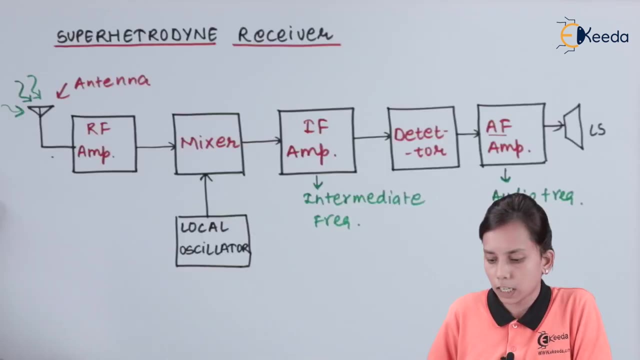 So still, we are not getting our desired frequency. So we will go back to our block diagram and we will try to find the answer Now. antenna is accepted, the frequency, So we have these various types of frequency, We have a tuned amplifier or this RF amplifier, radio frequency amplifier. 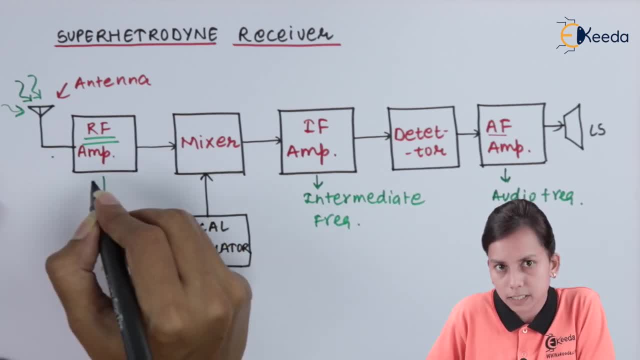 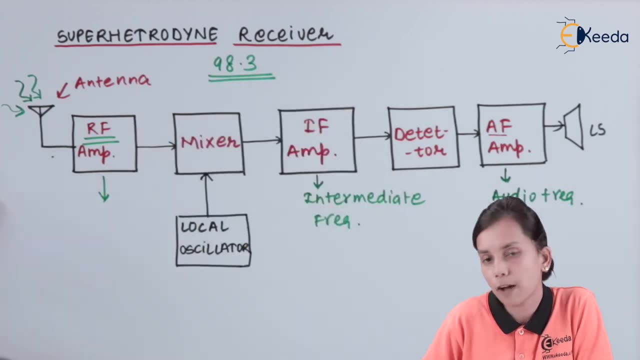 The working of this radio frequency amplifier is that if I want- let's say I tuned my radio at- I wanted to listen the music at 98.3.. Let's say this is my frequency of my station. So what our radio frequency amplifier will do, 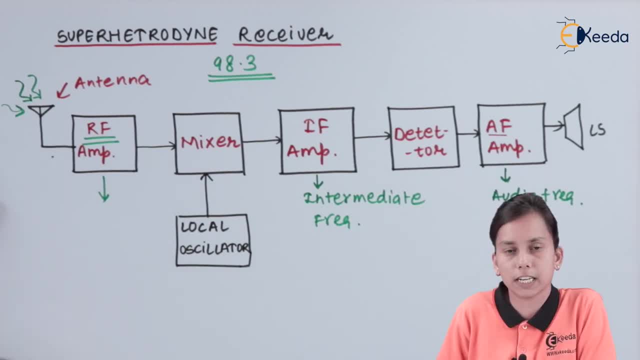 It will just select the desired frequency. It means that it will reject all other frequency and just accept that particular electrical wave, which consists of 98.3 frequency. Reject all the frequency and accept only 98.3 frequency. So what I can say. 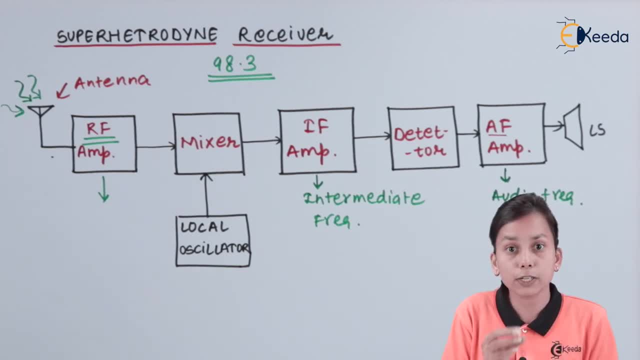 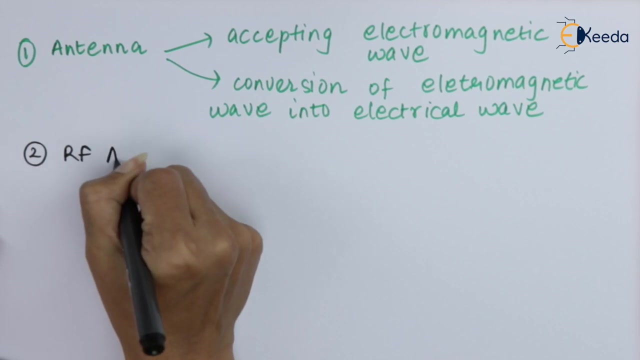 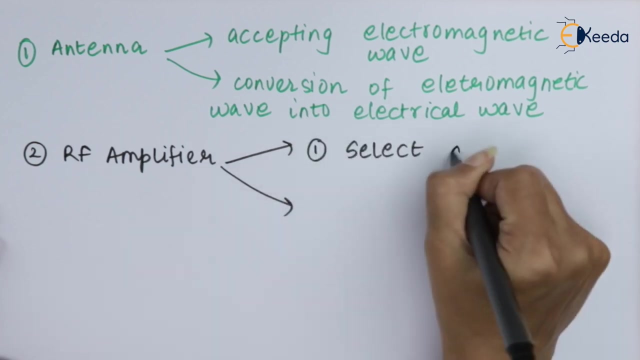 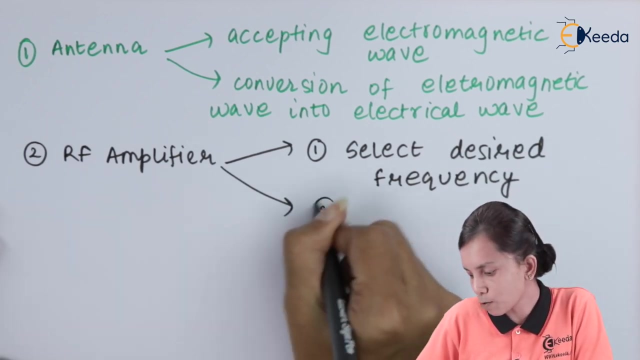 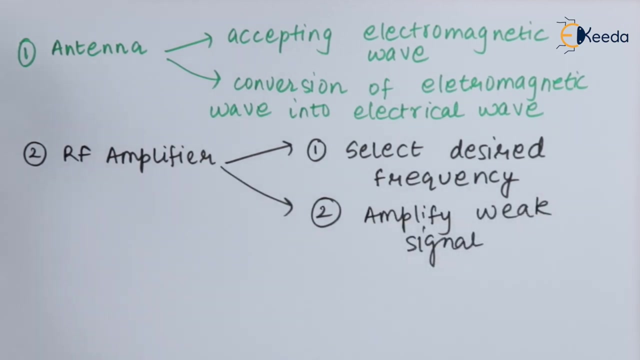 The working of radio frequency amplifier is to select the desired frequency. Selectivity of any frequency or the desired frequency is the working of our radio frequency amplifier. So let me note down this point: RF amplifier Select desired frequency. Second one: It also amplifier. 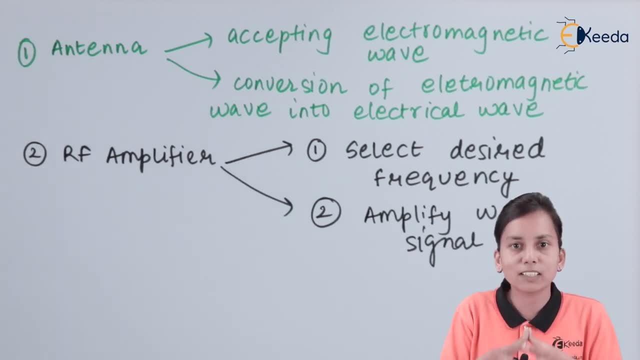 Though its main work is to select the frequency, but as it is also amplifier, So it will amplify our weak signal, that signal which already transmitted from a long distance, So it will also amplify our weak signal Now, After getting our desired frequency. Now our function is to process that signal. 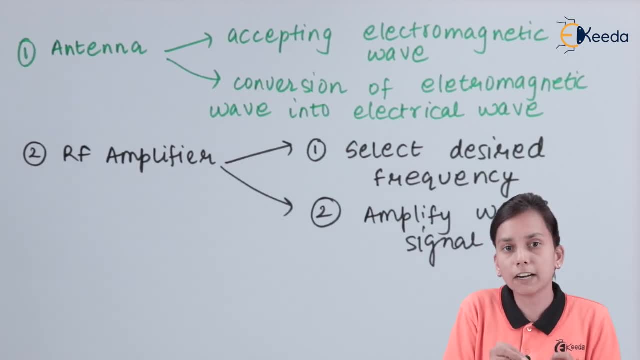 Because still it is not a form of a desired form. For example, if I am sending a voice signal, That voice signal is actually converted into electromagnetic wave, Then electrical wave, Still my main transmitted signal. It is supposed to be in the form of a voice signal or a sound wave. 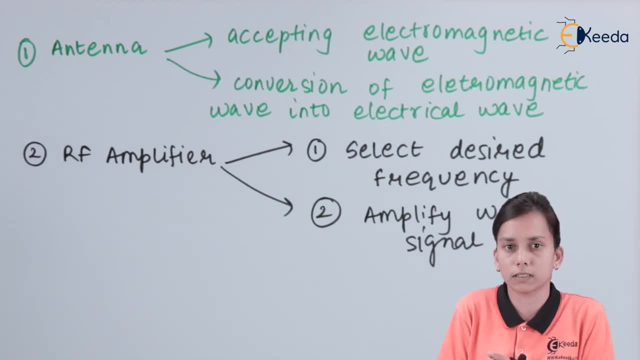 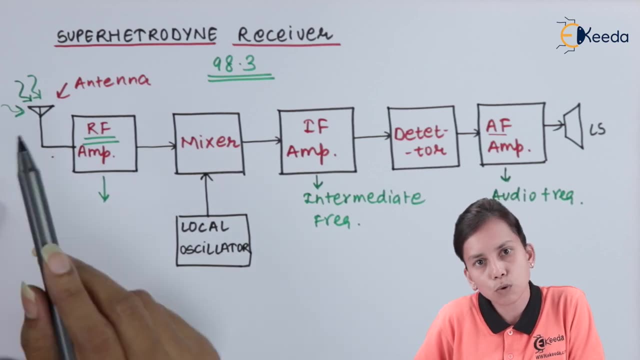 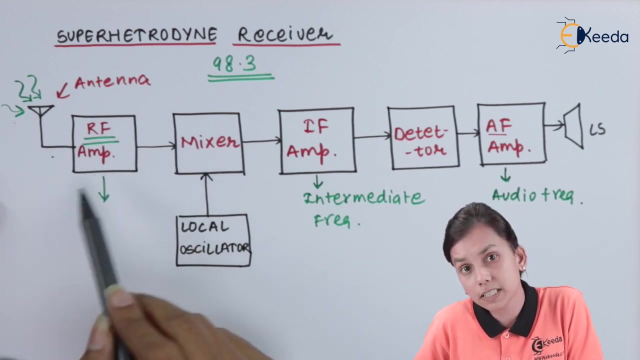 We are not getting a sound wave. Still we need to process it Further. So let us get the answer for this question. We accept the frequency of so many stations, Then we select our desired frequency. Now, desired frequency is a very high frequency. 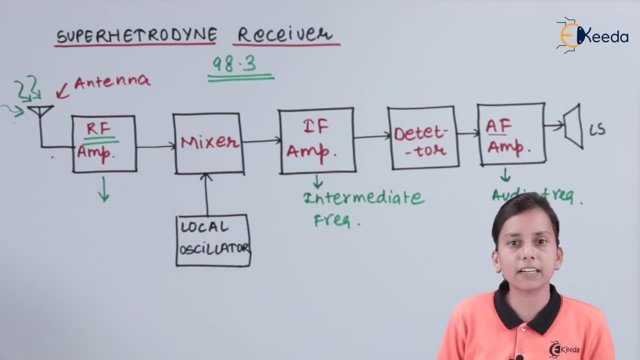 And we are not interested in a very high frequency. We are interested in a low frequency signal Which was actually transmitted by me During the whole process of modulation. So What mixer will do This third block? The mixer Will actually convert. 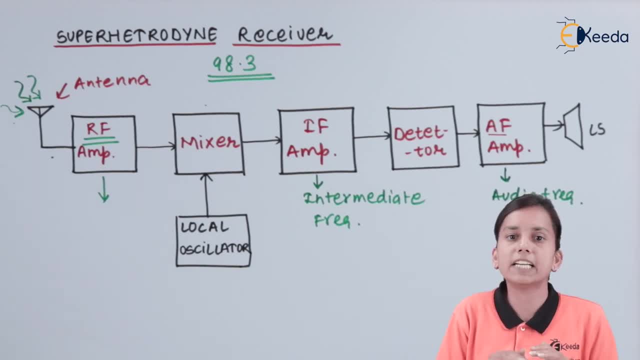 My desired frequency Into a medium frequency With the help of local oscillator. Local oscillator will produce some frequency, And we will actually. This is our mixer. Now mixer will get The frequency- Desired- frequency, As well as the local oscillator frequency. 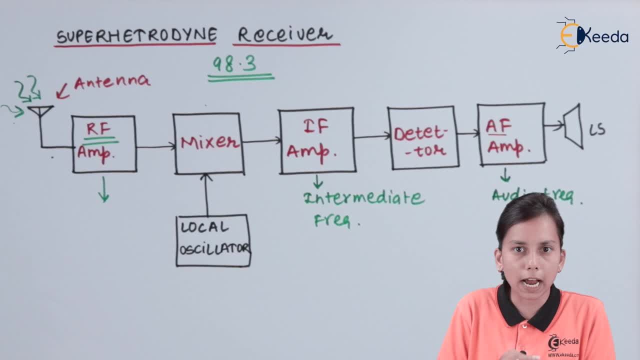 They will subtract a. They will also Adding of a frequency Or subtracting of this frequency. We will just get a Media frequency And that process actually known as Heterodyne. If I am converting A high frequency signal, 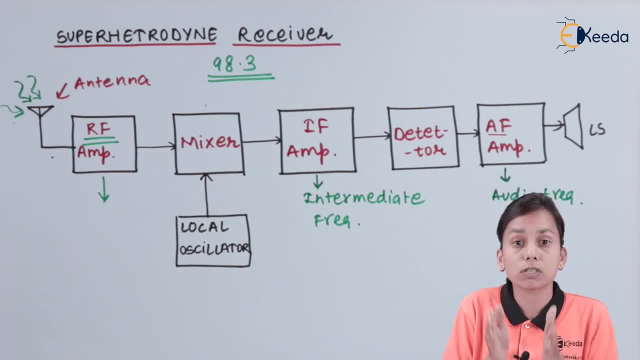 Into a mixed band frequency signal. That process is known as Heterodyne. That's why this receiver is also known as Super heterodyne receiver. That super heterodyne receiver Is Actually performing this Heterodyne process. 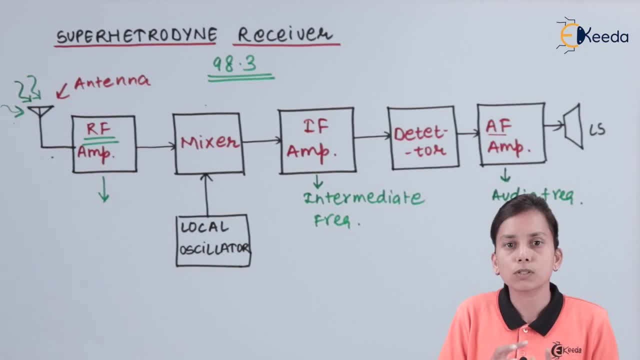 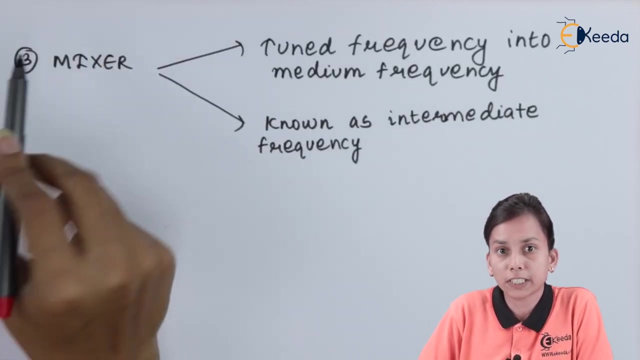 And heterodyne process is nothing But the difference Or addition Between the high frequency And the local oscillator frequency Signal, So that it is producing a medium frequency. Let me call this frequency as Intermediate frequency. So I have written down. 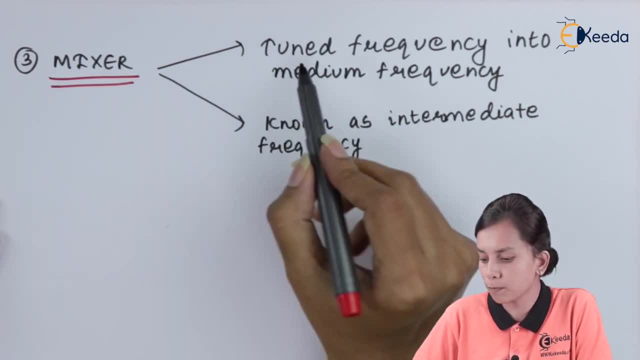 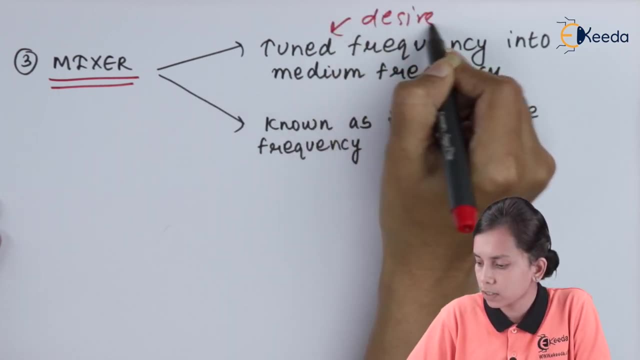 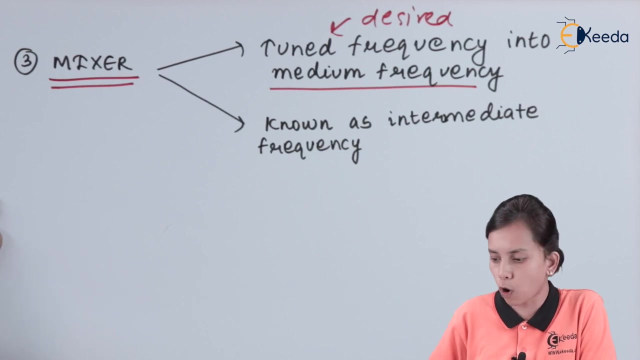 The working of mixer Is that, First, one Mixer is actually converting our tuned frequency- Tuned is Desired frequency- Into Intermediate frequency Or a medium frequency. First of all, Our mixer is actually converting The tuned frequency Into a medium frequency. 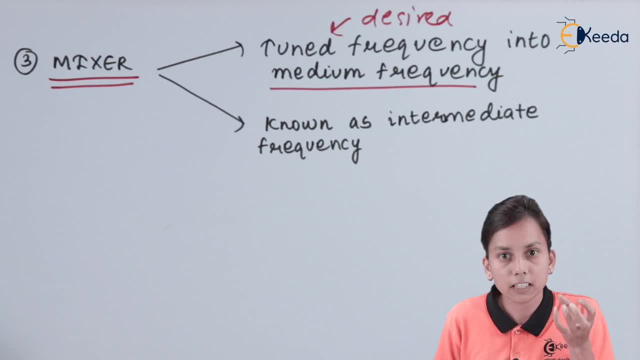 With the help of Mixing, And this mixing is doing With A local oscillator. Now What I am saying? that Instead of calling this as A medium frequency, I am using this term Intermediate frequency. This medium frequency Is known as: 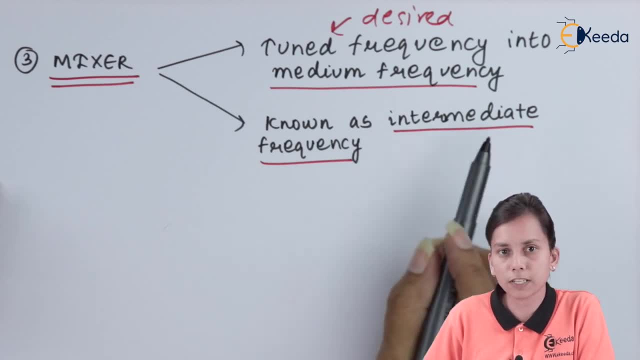 Intermediate frequency. So If someone is asking me to Explain The working of this mixer, So what We can say: That mixer Is actually performing The process of mixing By converting The tuned frequency Into the Medium frequency. 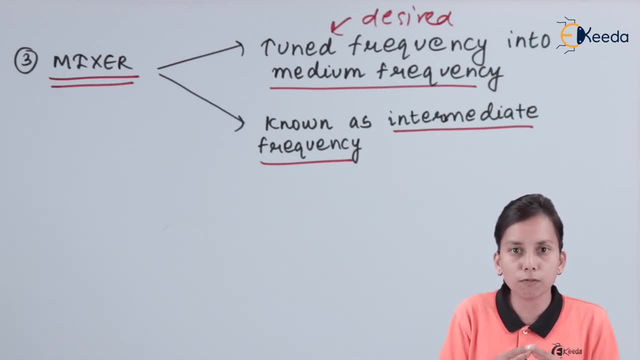 With the help of Local oscillator. Such a process Is also known as Heterodyne Process, And that Medium frequency Is also known as Heterodyne Process, And that Medium frequency Is known as. 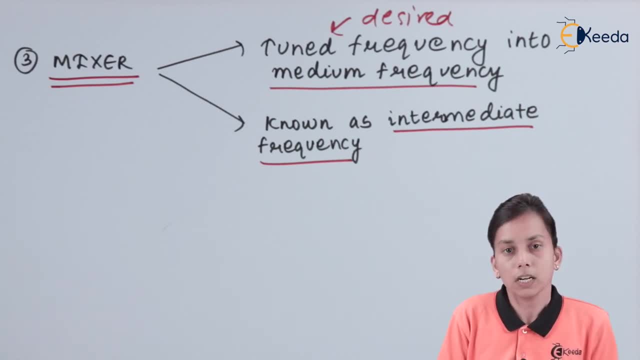 Intermediate Frequency. Now, If I am converting A intermediate Frequency, That signal Has to be Amplified. So For that Purpose We will have A new block, Which is known as IF Amplifier. 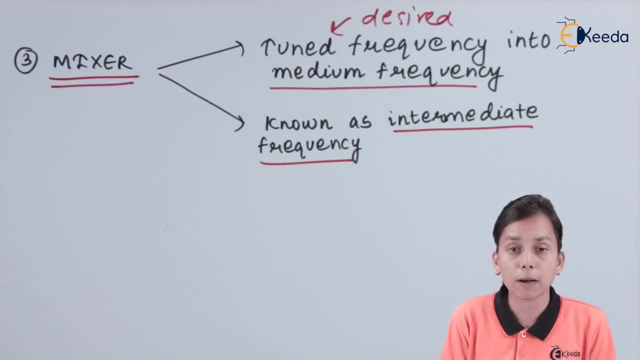 That is, Intermediate Amplifier. By introducing This IF Amplifier We can increase The selectivity Because Sometimes The Amplifier, Sometimes The selectivity Is get affected Because Of the noise. 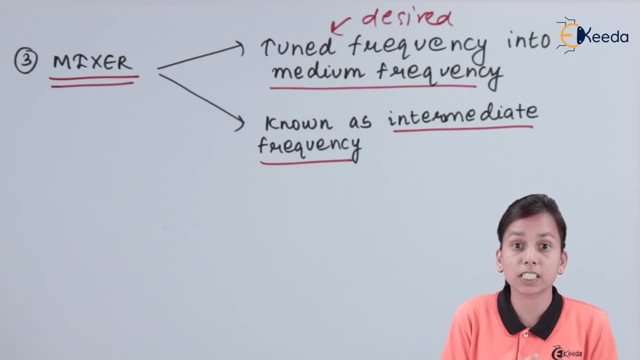 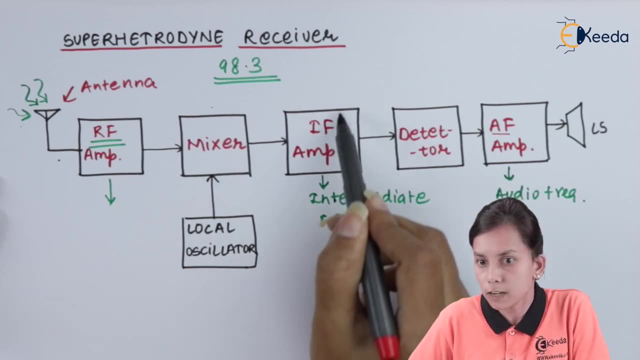 So This IF Amplifier Will ensure The more Selectivity, Sensitivity, Fidelity In our Communication System. So The intermediate Frequency Signal Will Amplify With The help Of this. 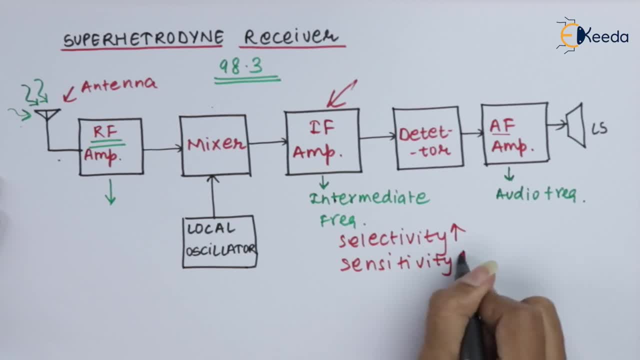 IF Amplifier And Fidelity Fidelity. Basically, We Are Actually Reducing The Interference, Or What We Can Understand By This Term. We Are Actually 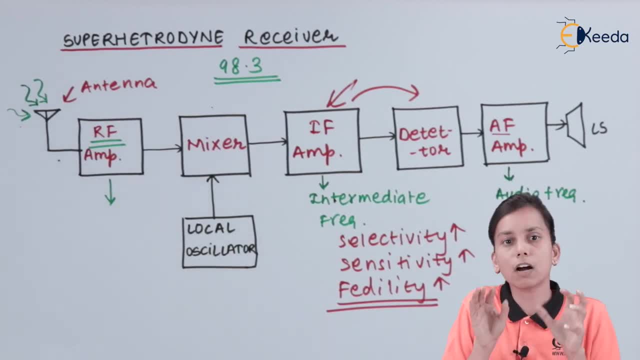 Reducing The Losses. That's It. So Next One: Now We Will Process Our Signal With The Help Of This Detector. Basically, Detector Will Perform. 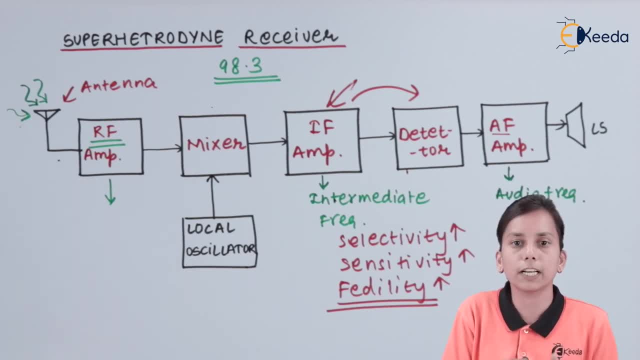 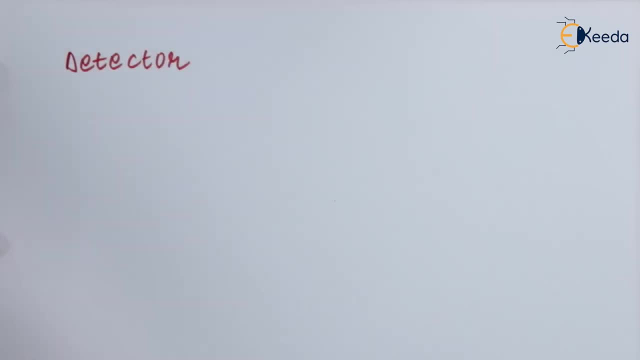 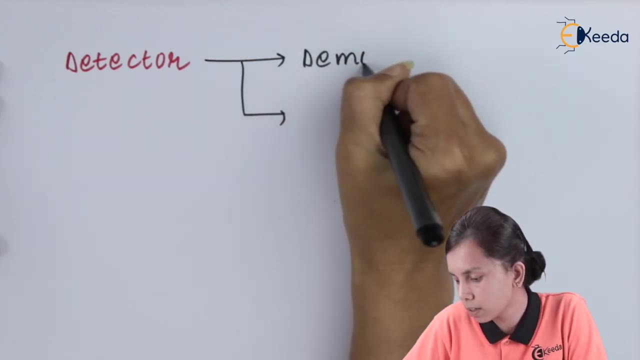 The Process Of Demodulation. Whatever Signal Is Actually Receiving, It Is In A Detector, Will Detect. So What I Can Say? It Will Perform. 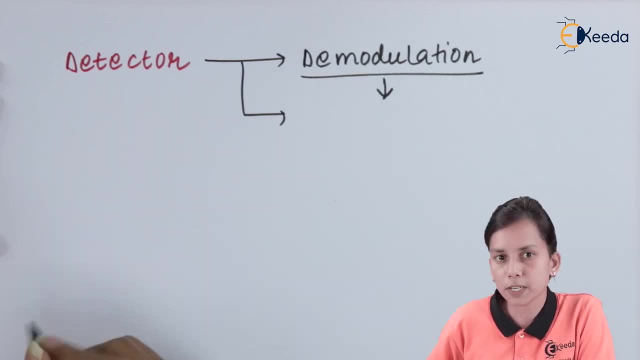 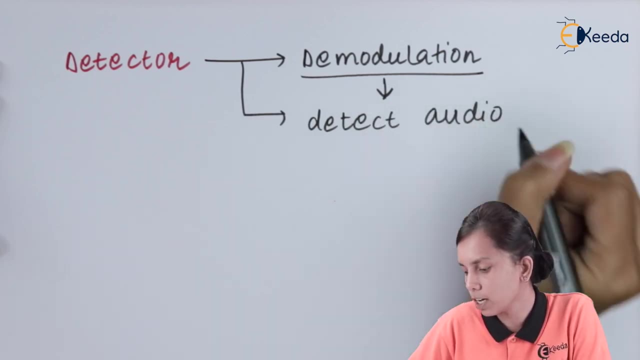 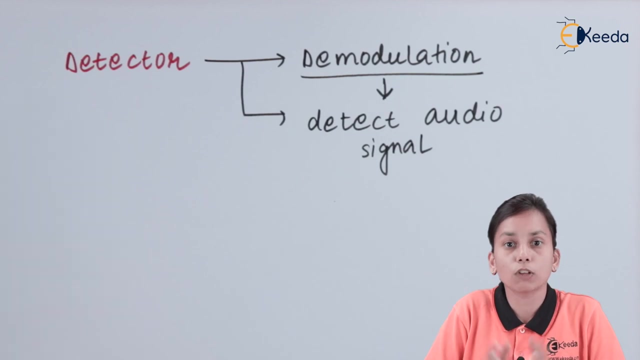 Demodulation And After Performing The Demodulation We Can Get Our Information. So I Can Say It Will Detect The Most Important Part Of The.